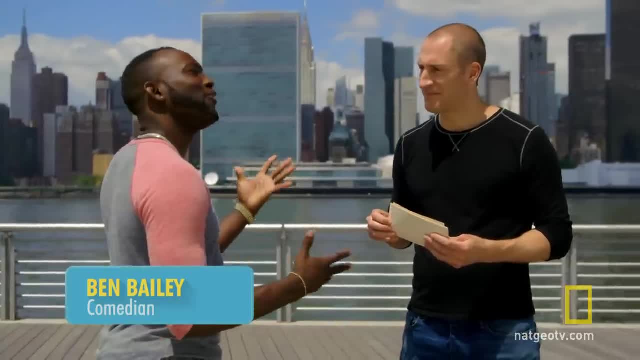 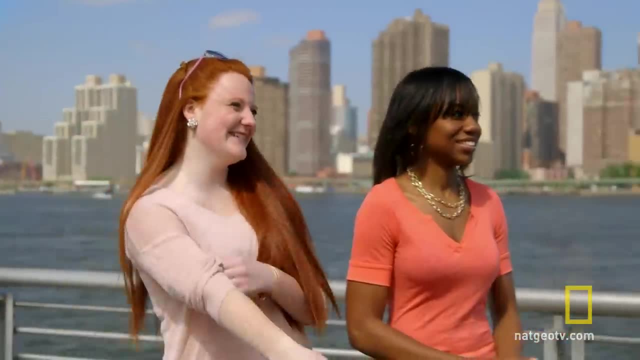 We've brought in comedian Ben Bailey to ask some people on the street a few logic questions. Play along and see if your common sense is better than theirs. Hello ladies, How you doing Good. Are you ready for the common sense quiz? Bring it on, Let's do it. 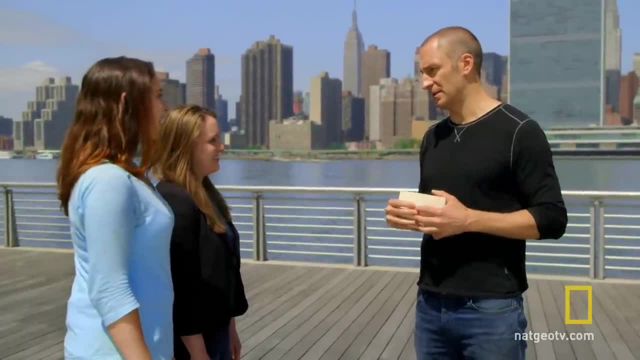 First question: do you feel like you're a person who has common sense? Not all the time, Not all the time, I guess. so That's a good, honest answer. More than average. Enough to get by. Enough to get by. 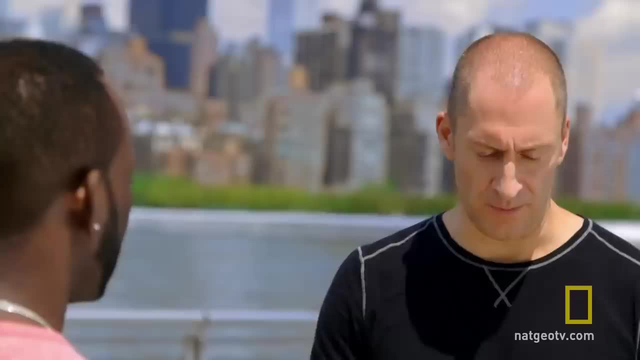 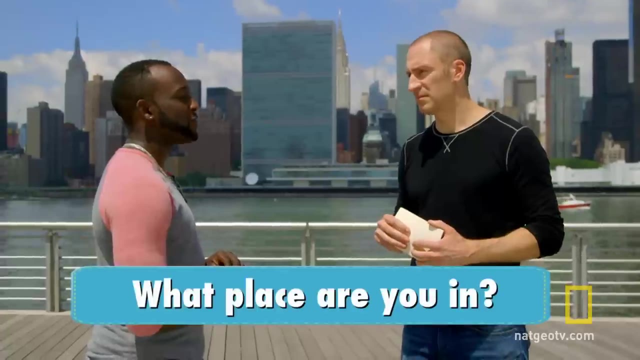 Yeah, Yeah. for the most part, We're about to find out. Here we go. If you're running in a race and you pass the person in second place, what place are you in? I know everybody said first. but am I going to be dumb and say first, 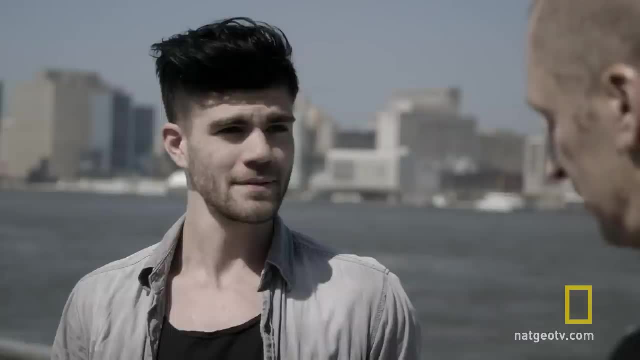 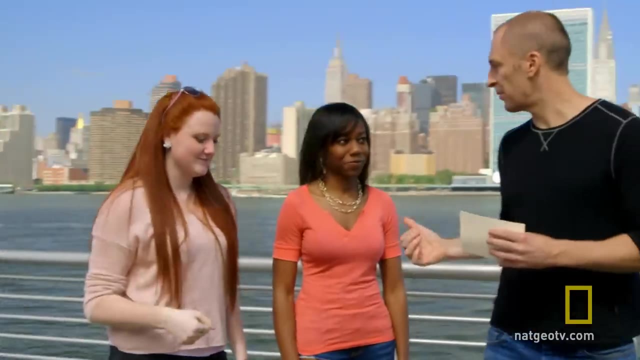 First, First, First. So what place would you be in? The answer: second place. I'm still stumped with that one. Let's pretend we're all in a race, You're in second place, You're in third, Then I'd be in second place. 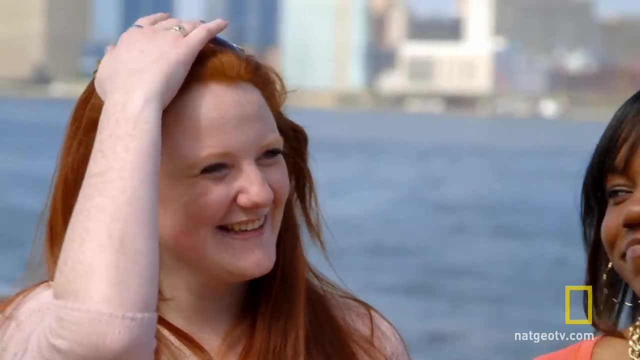 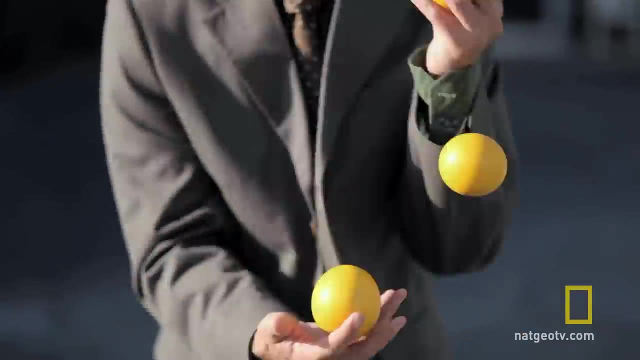 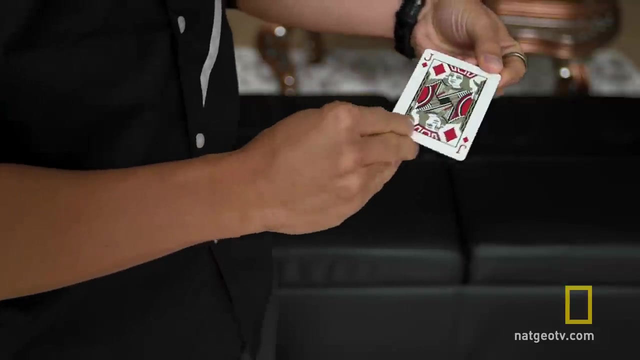 I'm winning, then you're in second place. Okay, I get it. Okay, Just me turning around did that? We admit these questions are designed to test your common sense, But you could also call them trick questions. So you'll have to pay really close attention and harness your uncommon sense to get the right answer. 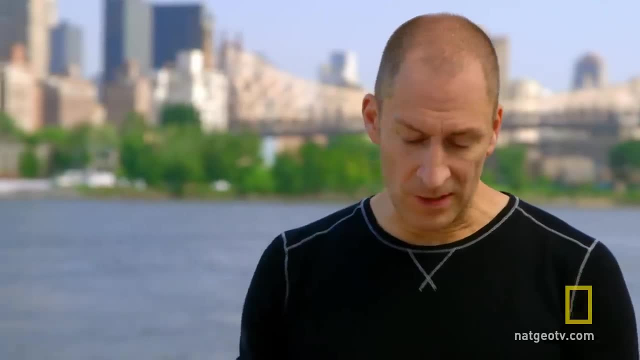 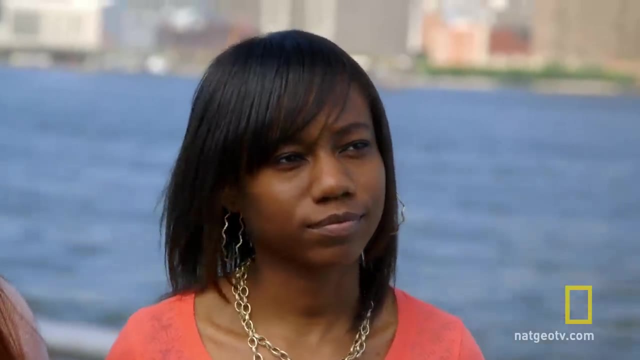 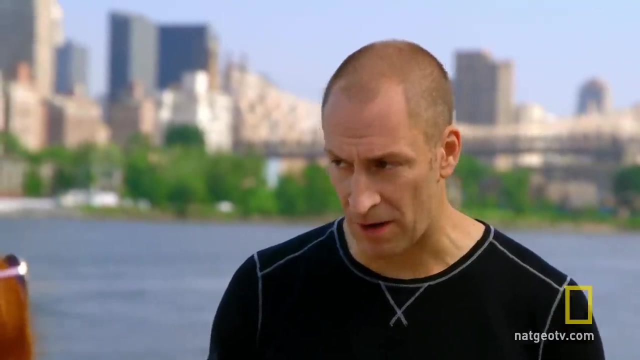 Think you've got what it takes. Of course You're driving a bus with ten people on it. At the first stop, four people get off and two get on. At the next stop, three people get off and five get on, And at the last stop, six people get off. 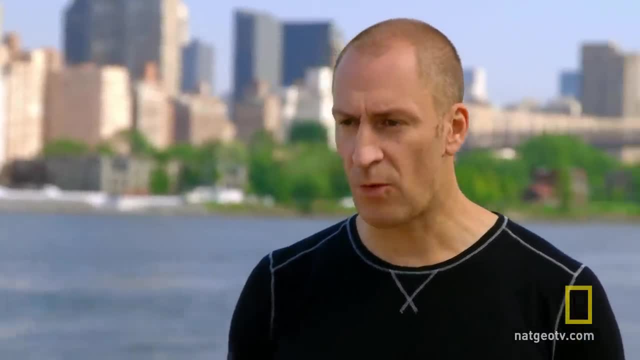 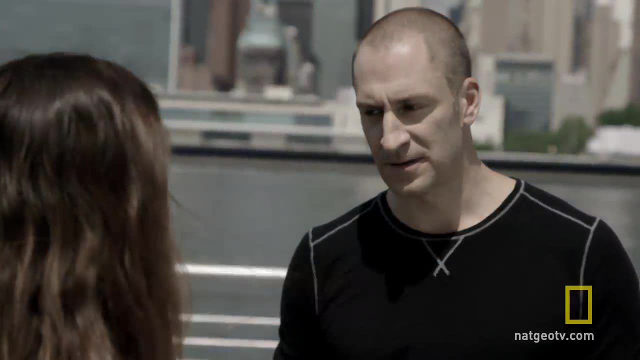 and only one gets on. How old is the bus driver? Give me a break. How old is the bus driver? That's a trick question. They're all trick questions. Do you have your answer at home? Old enough to drive a bus? 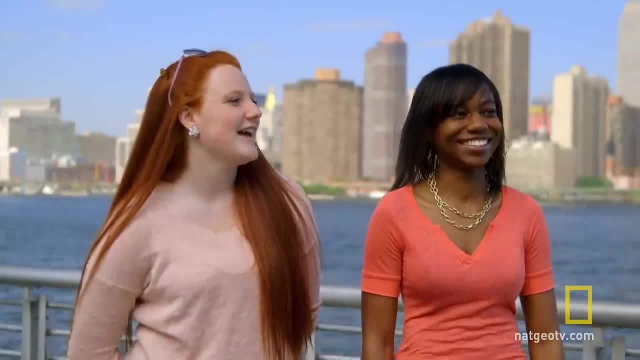 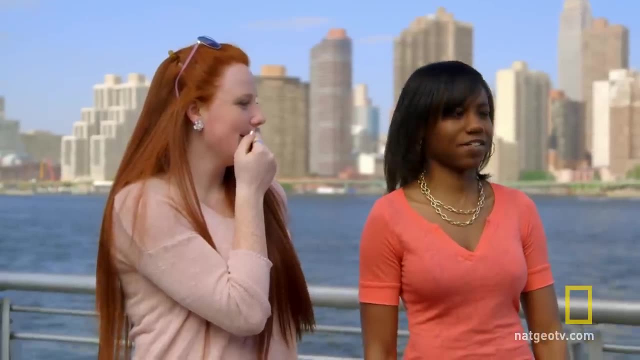 Sixteen Over sixteen. He is at least eighteen. He's at least eighteen. I'm going to say he's an older guy. He's an older guy About eighty-five, Eighty-five, Eighty-five. I'm not riding on that bus. 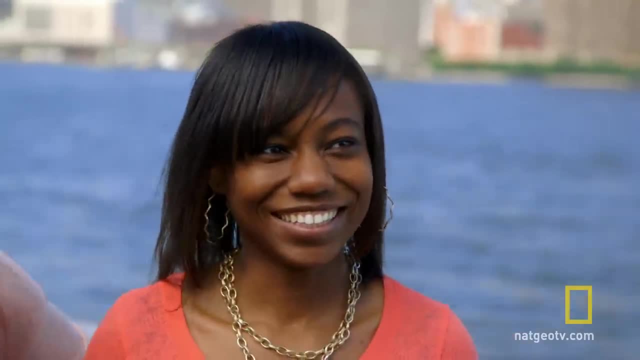 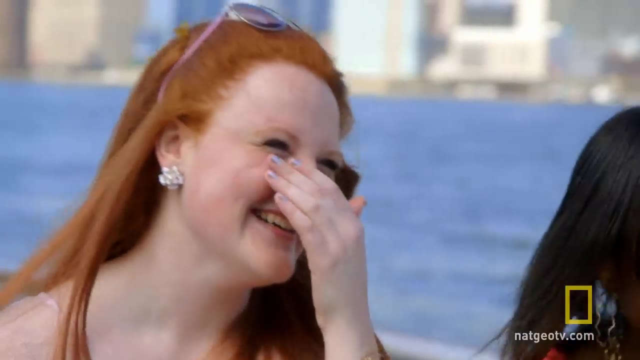 You're not riding. I think he needs to be retested. All right, I'm going to read the beginning of this question to you, and then you're really going to be angry. You're driving a bus, Oh no, Did you solve this riddle and give your own age? 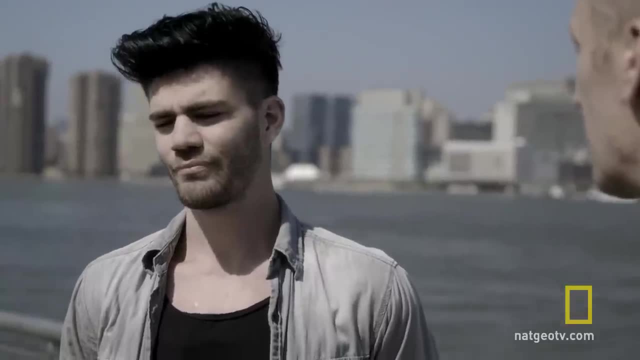 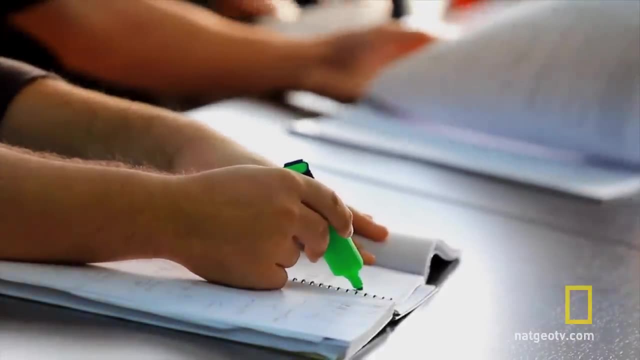 Hopefully you did better than our volunteers, But even if you didn't, it's not your fault. This test was meant to reveal how your brain trades facts for efficiency. When you're presented with a problem, your brain is naturally wired to use mental shortcuts to save time and energy. 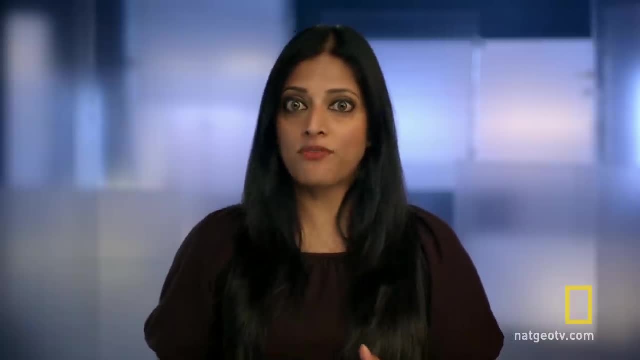 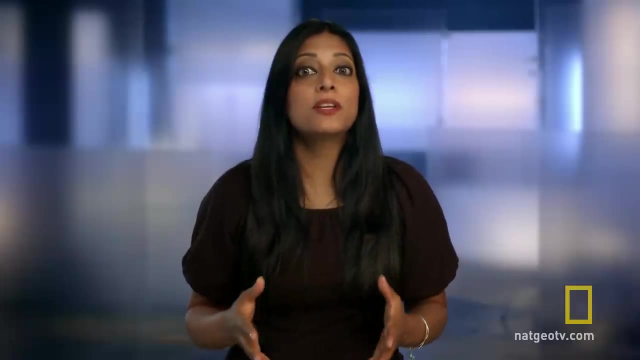 These shortcuts allow your brain to answer quickly and with confidence. The problem is that answering based on past experience, using what we call common sense, leaves open the possibility that you're incorrect, especially if your information is faulty or not up to date.